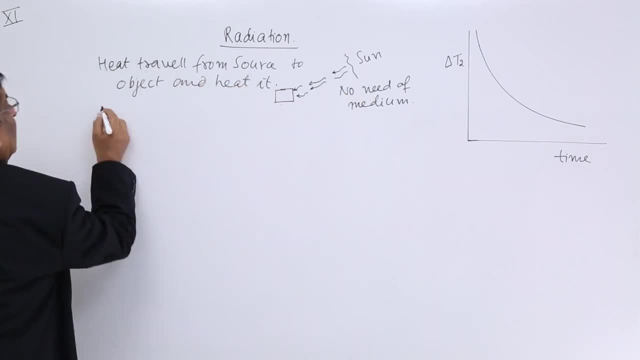 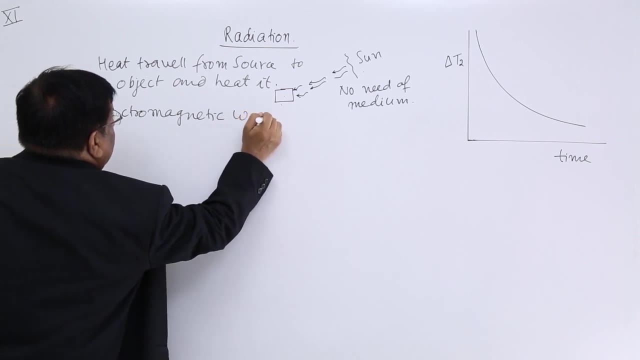 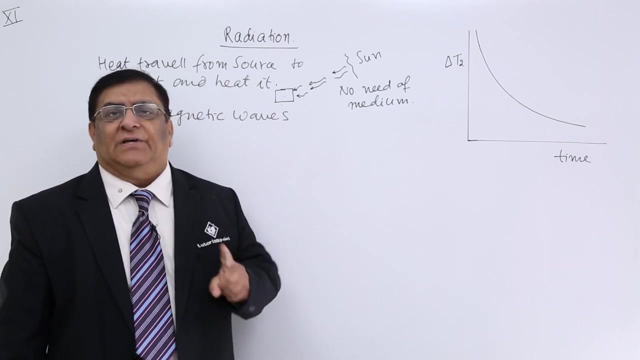 This is source, This is object and these are electromagnetic waves, Electromagnetic wave And this particular electromagnetic waves. there are so many types of electromagnetic waves, The one which are received by our mobile. It has been given the name radio waves. 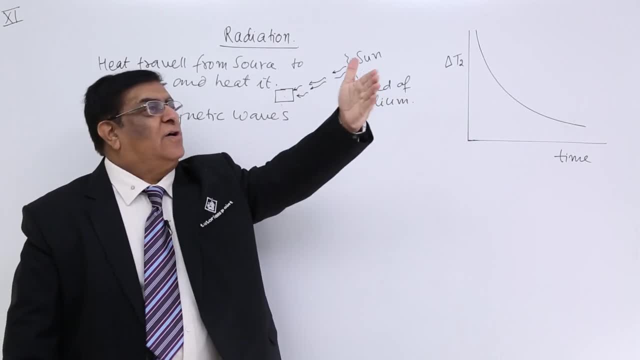 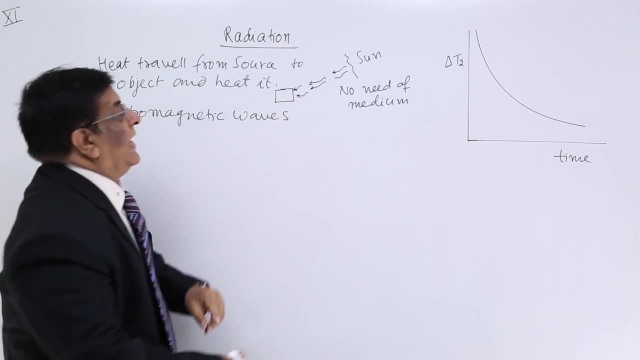 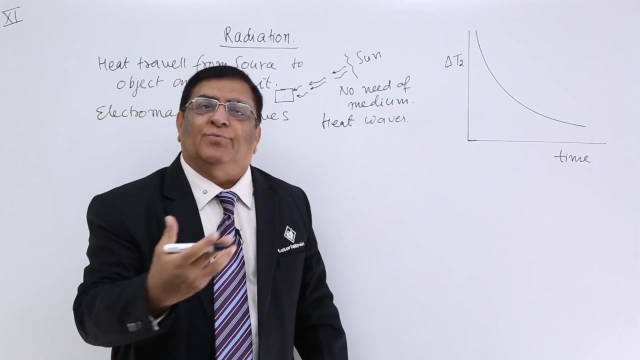 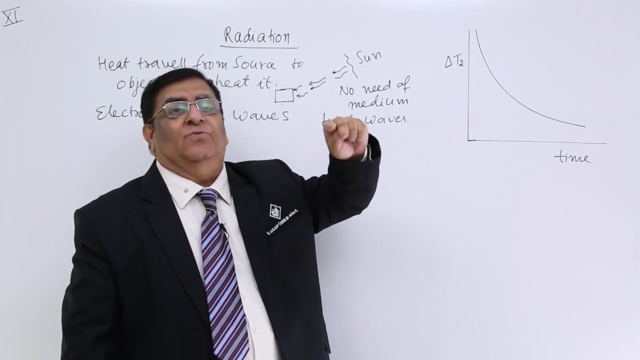 The one which are received by the mobile one through which we see the objects. those electromagnetic waves are light waves. The one which heats the object are known as heat waves, And there are other like x-rays and so many other waves, But all are electromagnetic waves of different wavelength that we will study in class 12.. 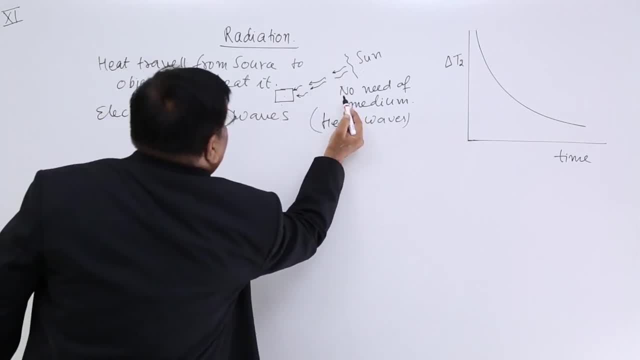 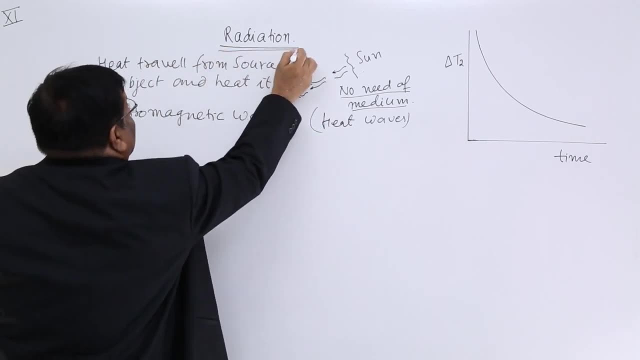 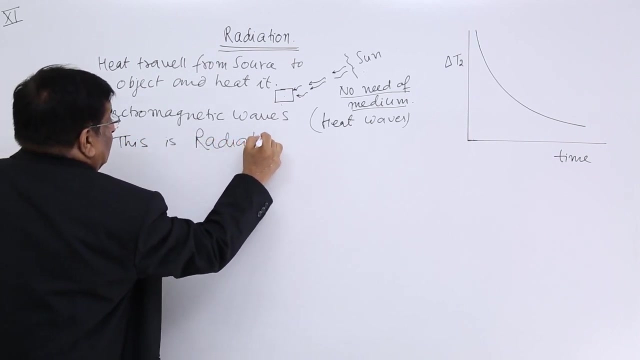 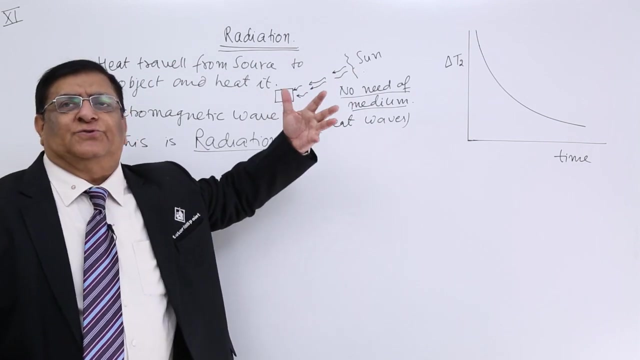 So these heat waves, they do not need any medium. This method of transfer of heat is known as radiation. This is radiation. Okay, In this radiation, when the heat comes here, there are so many different characteristics. We study. what does it do with the heat? 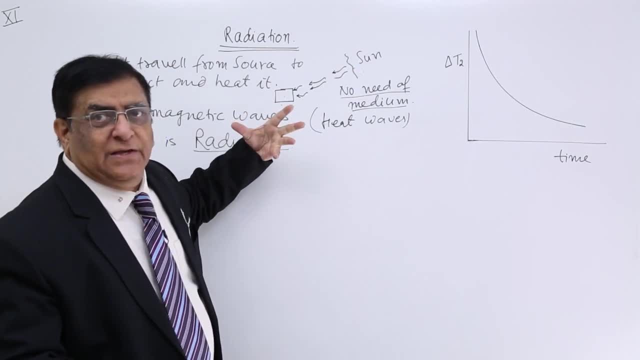 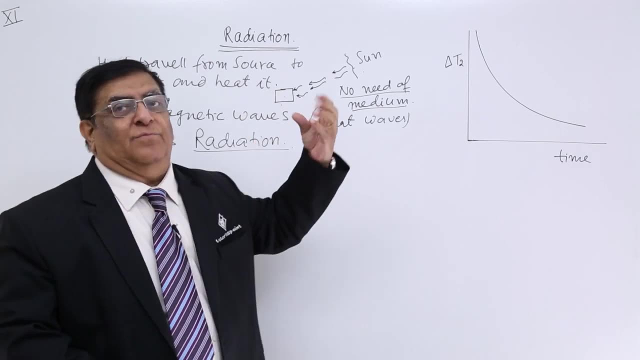 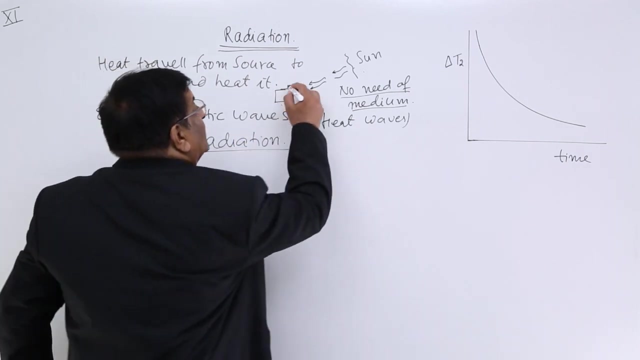 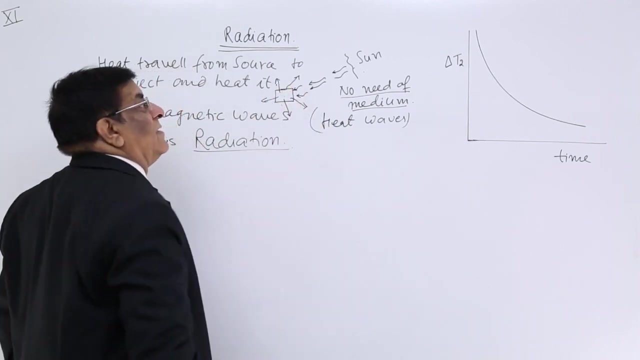 It received the heat, its temperature goes high and, with respect to these particles in the neighbourhood, its temperature become higher. When it has a higher temperature, it also starts radiating the heat. So it is also radiating the heat this way. So it is receiving heat from here and it is radiating heat outside. 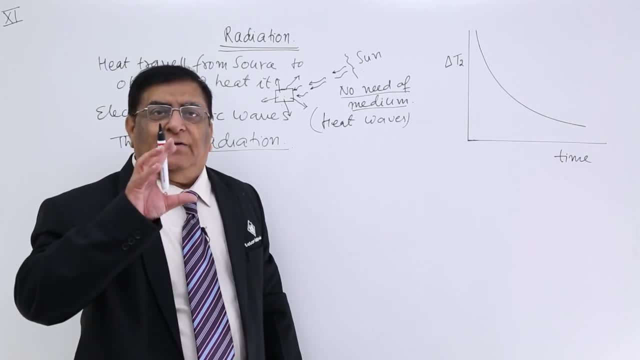 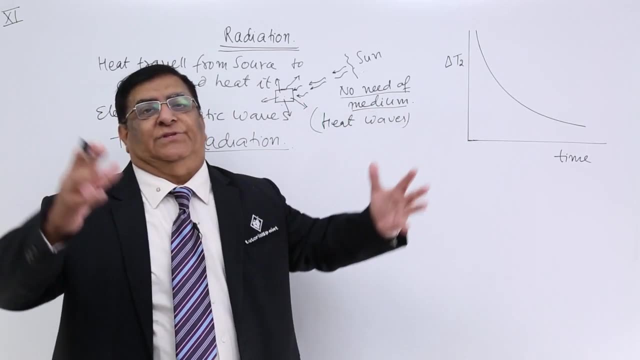 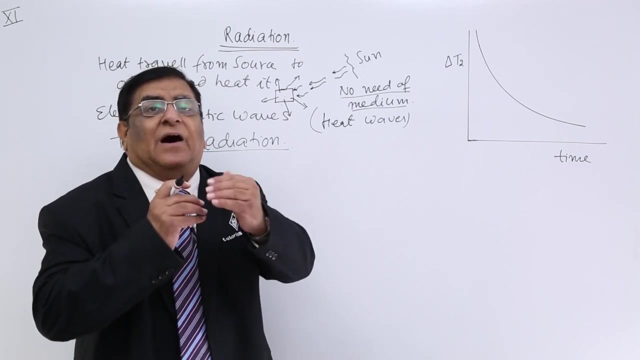 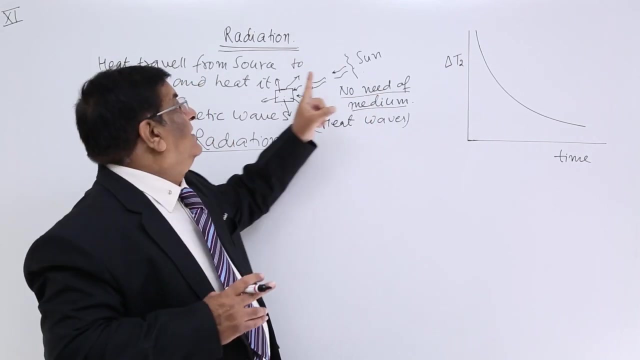 So what is the rule of radiation? A particle, a material which has a temperature higher than the surrounding will radiate out the heat. All the bodies which have got certain temperature are radiating out the heat. If their surrounding is hotter, Then they radiate out the heat which is less. they receive the heat which is more. So they get heated up. If in the night this source is not there, then they are only radiating the heat and they get cooled down in the night. But all 24 hours all the materials are radiating out heat because their temperature is higher. 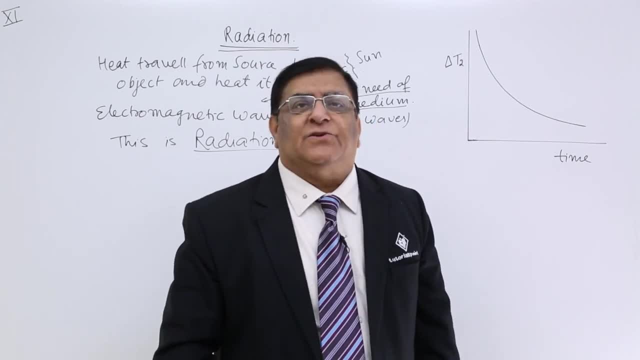 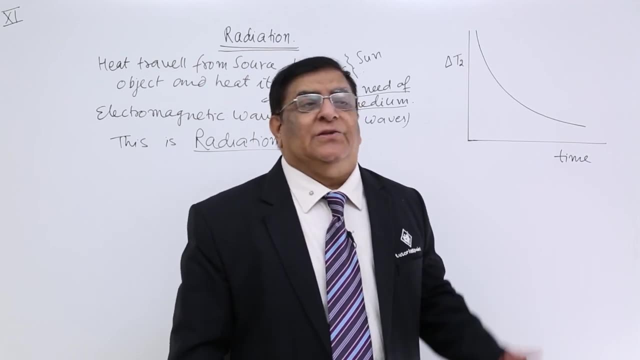 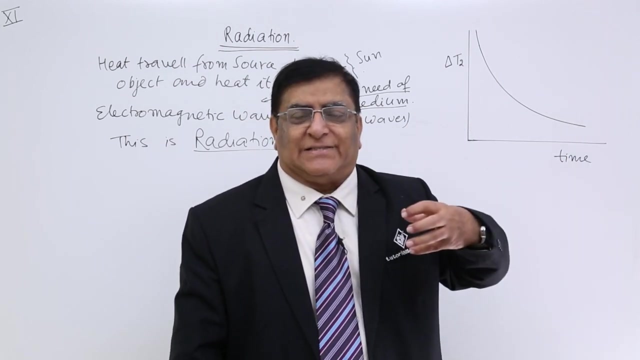 than the atmosphere. Even if it is not higher than the atmosphere, they are radiating out the heat. Mathematically we can say: they radiate less, receive more. they get heated up. If they radiate more and receive less, then they get cooled down. 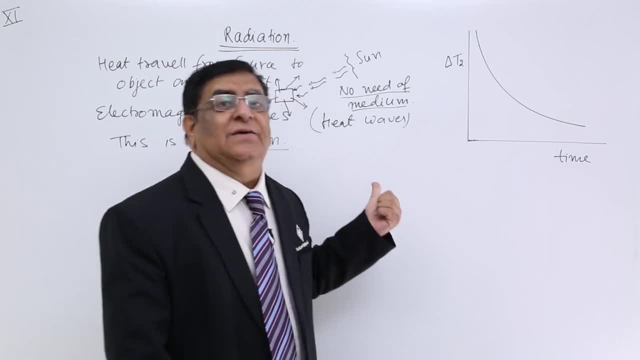 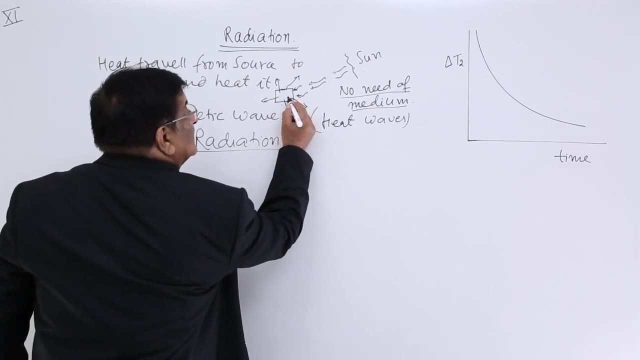 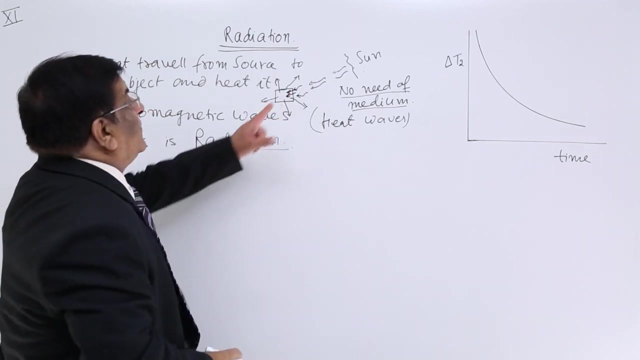 So this is cooling and heating of the material with radiation. So this method is radiation When it absorbs. This heat is being absorbed And going on And because of this absorption of heat its temperature goes high. The absorption is more and the second radiation is less. 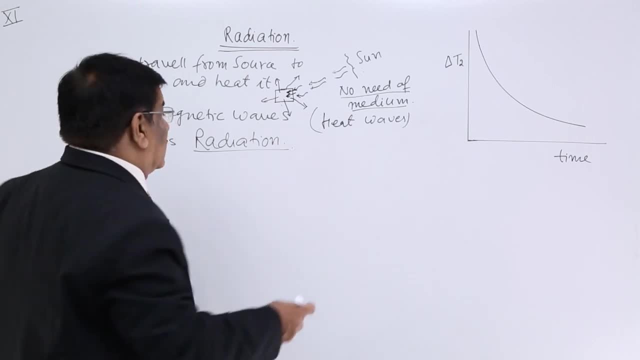 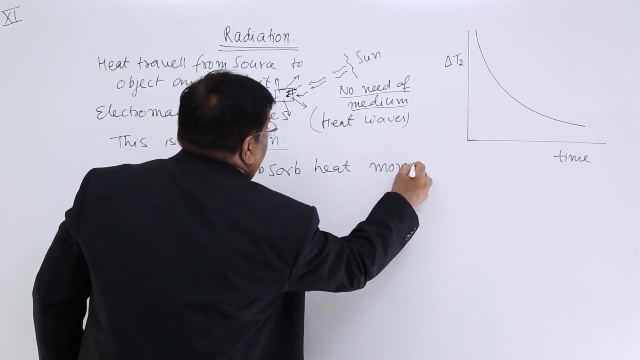 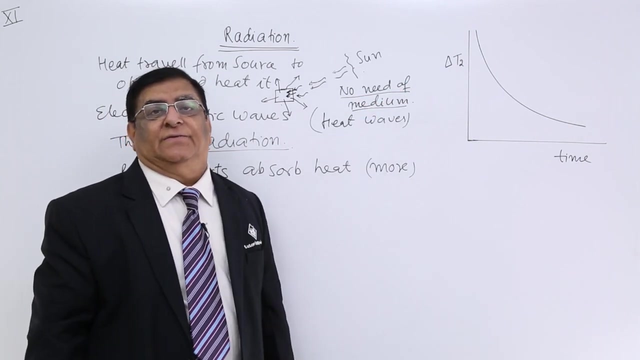 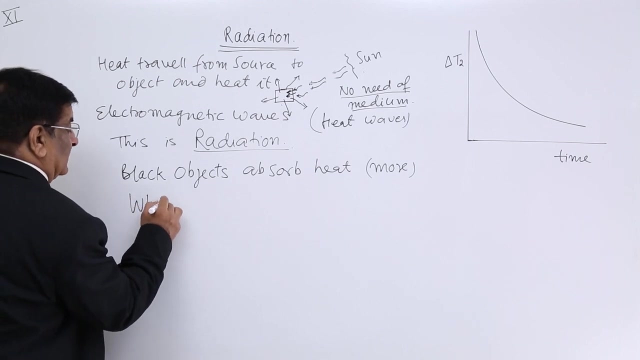 So it will get heated up. Who does this Answer? the black objects absorb heat more. If there is a perfect black, then it will absorb all the heat coming to it and will not radiate any Opposite to this- white objects. white objects absorb minimum. 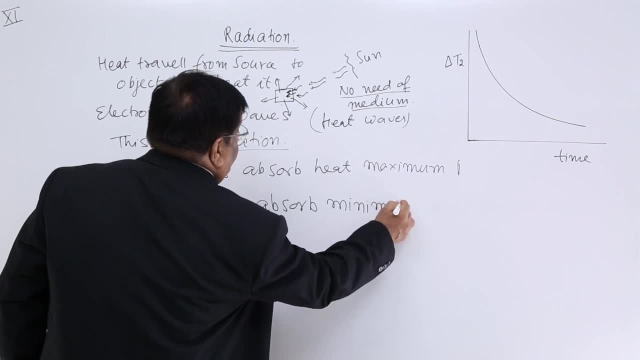 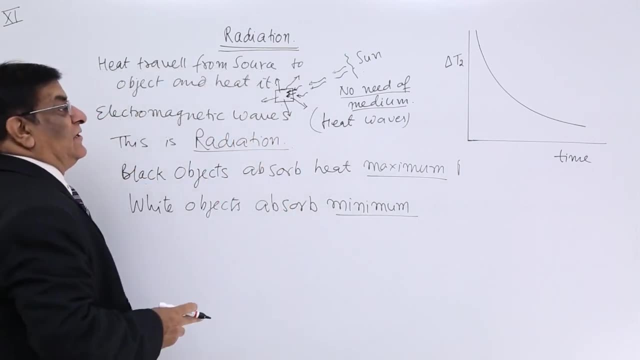 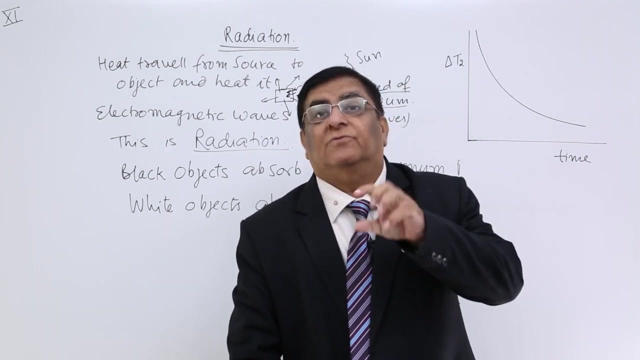 Absorb maximum. So this is the rule about it. For the radiation, we will further study. The object which absorb most will also get heat. In the same way we will study the black objects will also radiate most. It is this way. 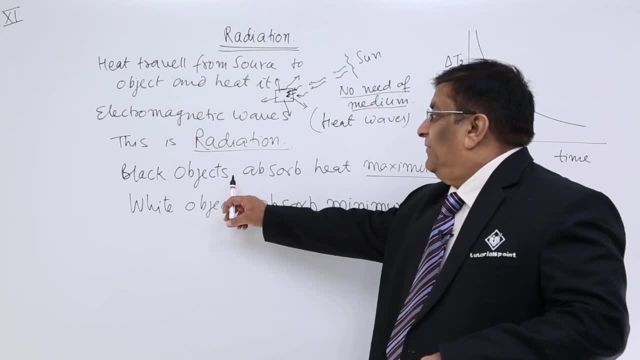 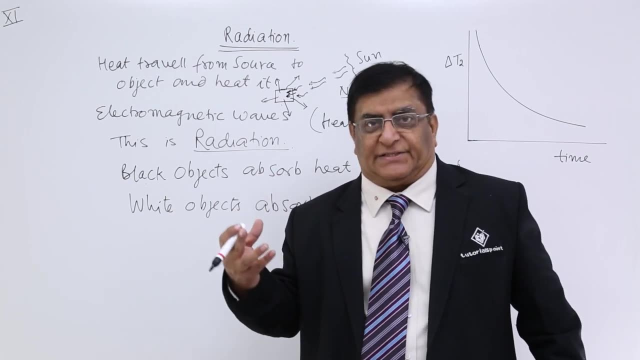 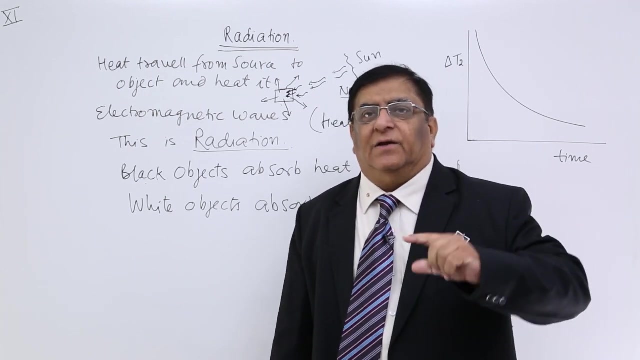 So when we want to radiate heat then there are different colors according to different temperatures for radiation of heat. Those are the different rules. we will study in that. But here, when we get the radiation from the sun, radiation of the heat, which color absorb most? 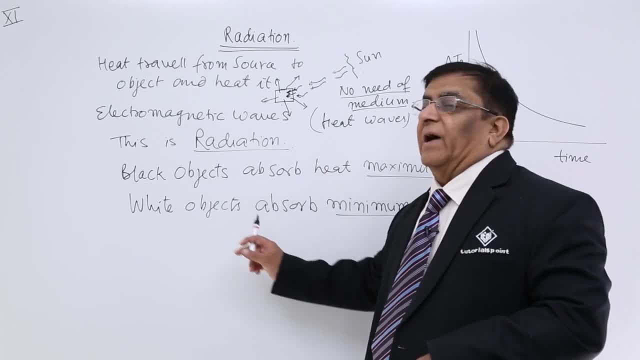 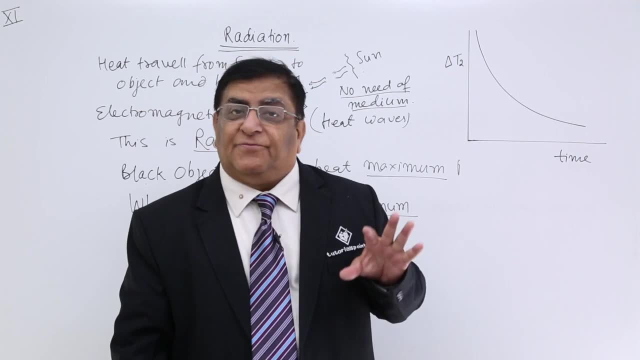 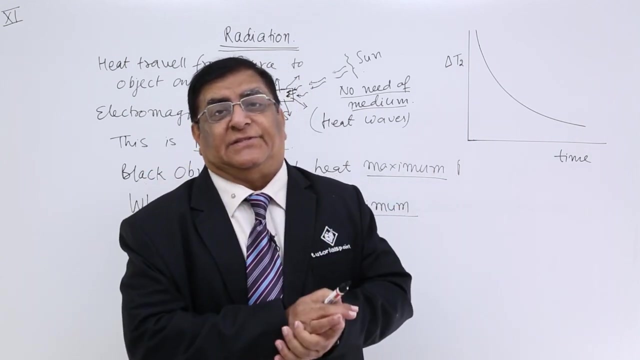 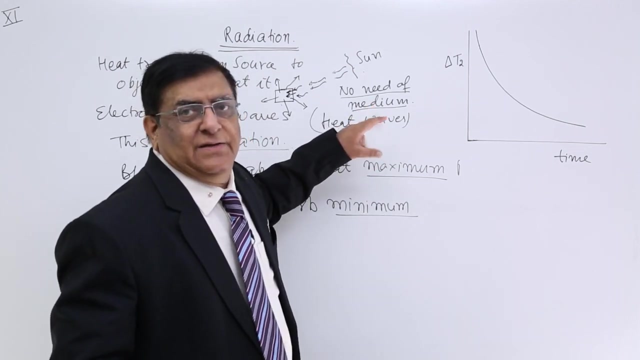 Black absorb most and white absorb minimum. That's why in summer we use white clothes maximum, and if we have black clothes in summer, we feel very hot because it will absorb the heat and keep it with itself. So this is radiation. Now we do not need medium in that.